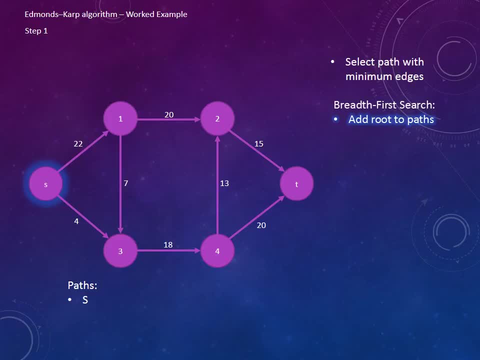 The first stage of this is simply to add the root node to our collection of paths. Now that the root node has been added to our collection of paths, we have to inspect the children connected to it. For example, the two children nodes are 1 and 3.. 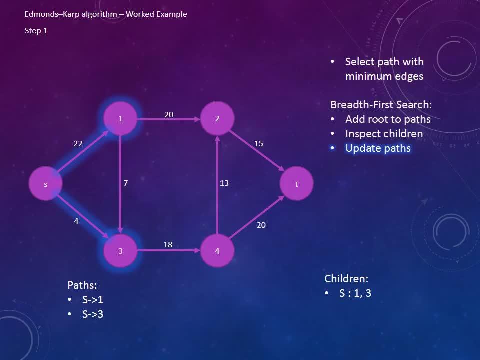 So we note that and then update our collection of paths so that we now have s to 1 and s to 3.. Now we need to inspect the children of the ends of the paths that we currently have. So the children of 1 is 2 and 3 and the children of 3 is just 4.. 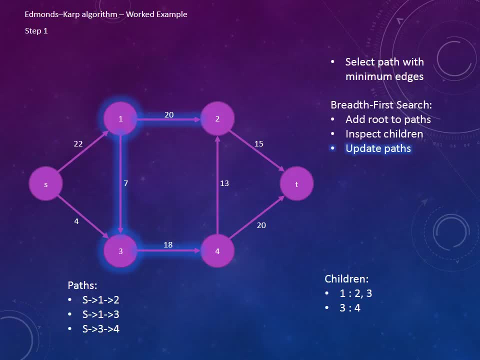 Okay, so now we need to update our paths again. s to 1 can also go to 2, or it can go to 3.. So we need to note that and make them two separate paths in our collection of paths. Meanwhile, s to 3 can only go to 4.. 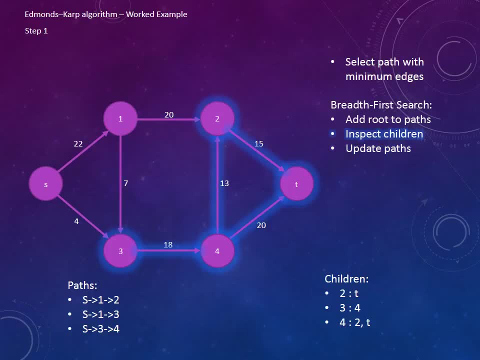 And now, finally, we just need to check the children of the paths that we currently have. So from 2, we can get to the sink straight away. So congratulations, the algorithm has terminated, Now that you've finally found a node that connects to the sink. 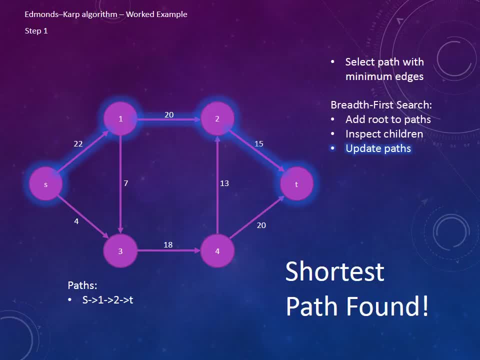 we can go back and update our paths accordingly so that we have a path from source to sink. The shortest path has been found. Now we'll discuss the rest of the algorithm. The first step is to select the path with the minimum edges. 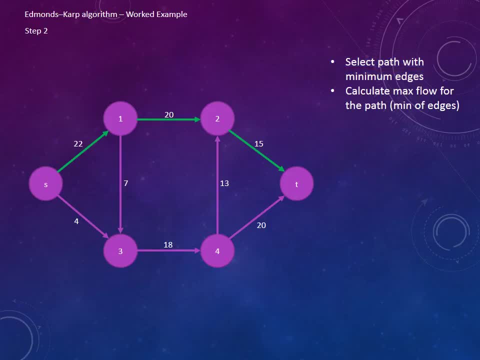 which is done via the process just shown. The next step is to calculate the maximum flow for this path. This is done by finding the edge with the minimum value. In this case, the edge with the minimum value is 15.. Now we need to update the residual graph. 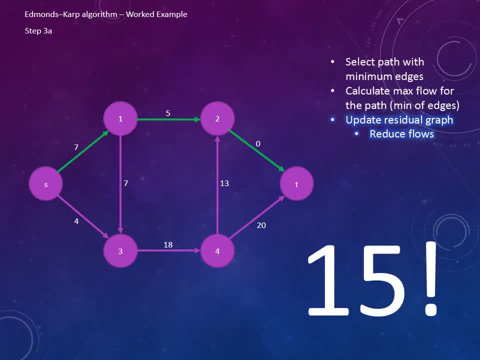 s to 1 is reduced from 22 to 7,, 1 to 2 from 20 to 5, and 2 to the sink goes from 15 to 0.. Now we need to add return edges. These are edges flowing in the opposite direction. 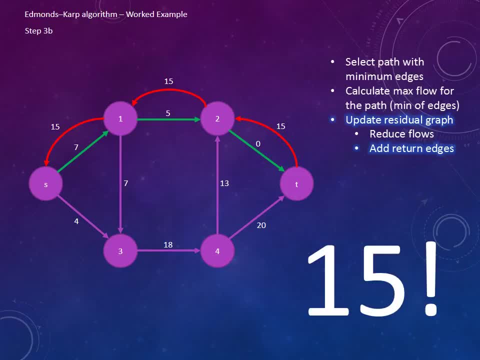 for the amount that we previously calculated. I like to think of these edges as a way of saying: we have pushed 15 that way, but we can decide to bring it back if we choose to, Now that we've allocated 15, to flow down this path. 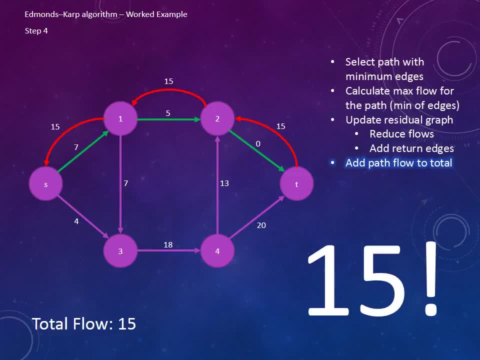 from the source to the sink. we can add 15 to the total. Notice the edge between 2 and the sink is now 0. It will be ignored in the next iterations as it has already got the maximum flow flowing down it. Some implementations choose to remove it. 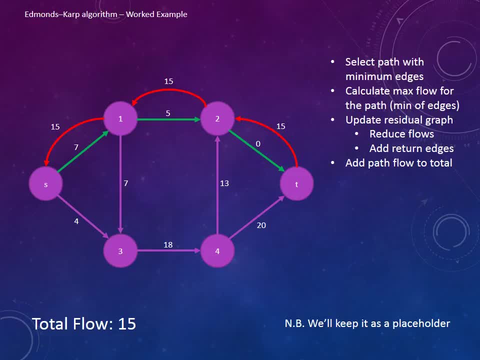 but for clarity, we're going to leave it there as a placeholder. Now we start the whole process again by selecting a new path with the minimum edges. The breadth-first search has chosen this one, highlighted on the bottom. Now we need to calculate the maximum flow for this path. 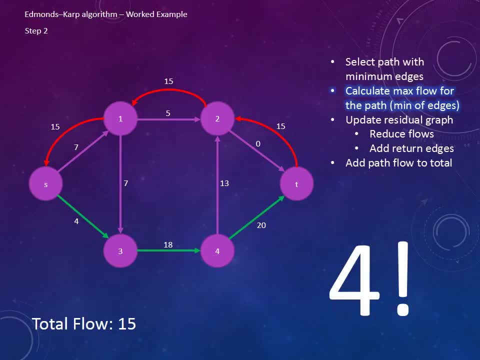 which, as you remember from before, is the minimum of all the edges, in this case 4.. Now we update the residual graph by reducing the flows by 4, and then add return edges for 4 back along the same path Now as we have allocated 4 to flow. 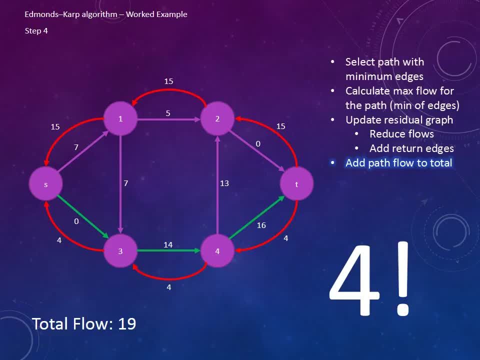 from the source to the sink, we can increase the total flow by 4.. Now we go back to the beginning and select the next path with the minimum number of edges. This is the path we have chosen. We now calculate the maximum flow of this path. 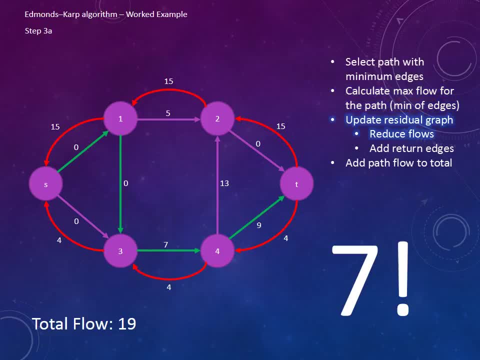 which is 7.. Now we need to update the residual graph by reducing the flows and then add the return edges. Now, as we have another 7 flowing from the source to the sink, we can add 7 to the total flow, As all edges from the source are maxed out. 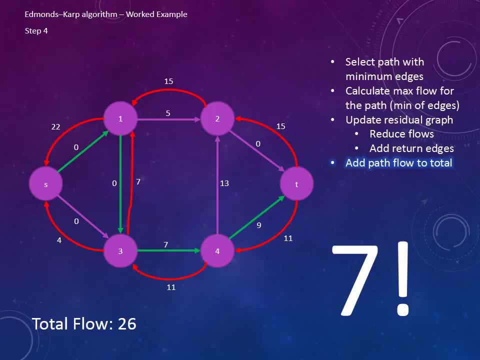 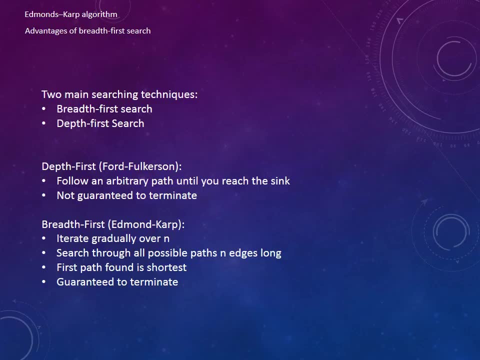 the algorithm terminates with a total flow of 26.. Like we mentioned before, there are two algorithms we can use to select the path in our max-flow problem. The first, which we have already explained, is a breadth-first search. This means it is an Edmund Carp algorithm. 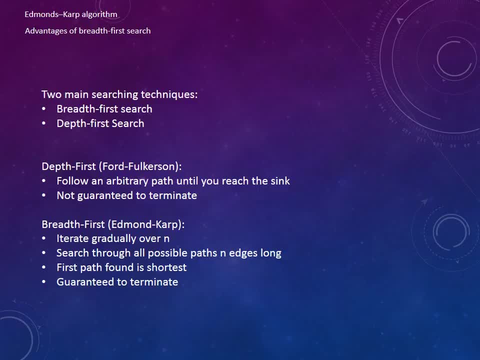 However, if we use a depth-first search, it becomes a Ford-Fulkerson algorithm. There is a disadvantage to the depth-first search: It is no longer guaranteed to terminate. We will explain this in further detail. Now we are going to solve our max-flow problem. 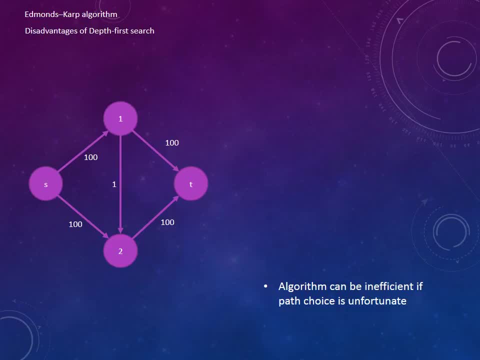 on this example: simplistic network using depth-first search- We are going to highlight why the Edmund Carp algorithm is truly the superior method. Again, we are going to select the path from the source to the sink, But now notice, it is an arbitrary path. 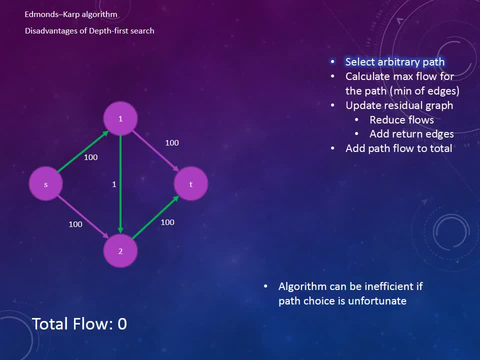 not the shortest path, like before. Now we are going to calculate the maximum flow of this path. Now we are going to calculate the maximum flow of our selected path And then update the residual graph with the new capacities And, of course, add the return edges of 1.. 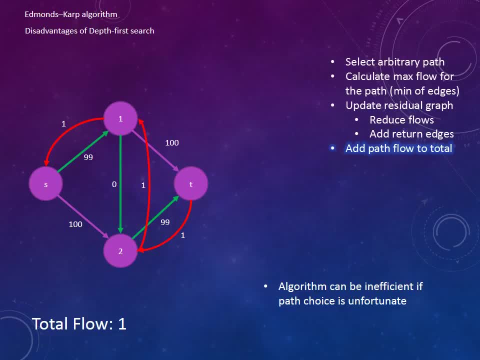 Now, that is all done for that path. Now all we need to do is update the total flow And again select another arbitrary path. Now we need to calculate the max-flow for this path, which also happens to be 1 again. Now we need to reduce the flows of our selected path. 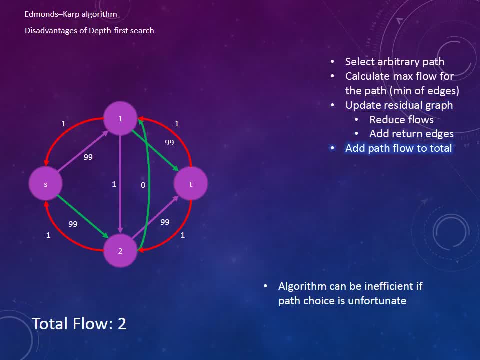 And now update the return edges And now update the total flow to 2.. Continuing onwards, we need to select yet another arbitrary path. The algorithm could just happen to select the same one as before. That is completely fine, because it is still a valid path. 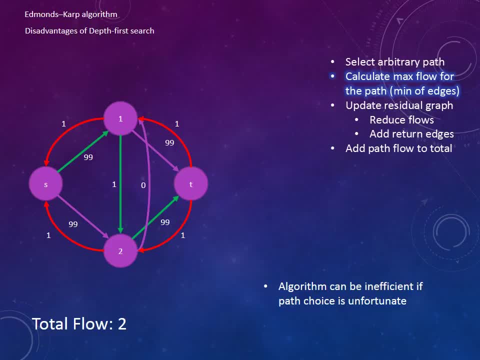 Calculate the max-flow of that path. We have got 1 again And update the residual flows. Now we have gone from 100 to 98. And, of course, update the return edges to 2.. Now again, add 1 to the total flow. 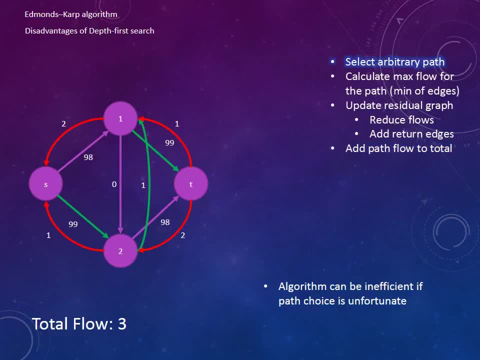 Now we are going to start the process again, selecting another arbitrary path. Now we are going to calculate the max-flow of that path And update the residual graph with the reduced flows. Add the return edges, updating them all to 2.. And now update the total flow to 4.. 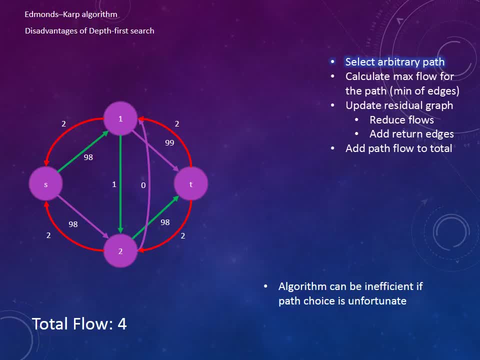 Again selecting an arbitrary path. Again calculate the max-flow for this path, Update the residual flows, Add the return edges And update the total flow to 5.. Now you can probably notice a pattern. now It is very slowly iterating through the algorithm. 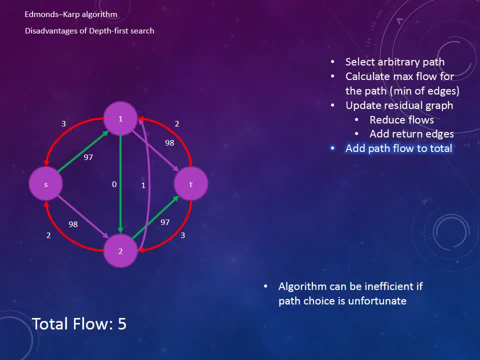 taking 1 off the path at each stage. Now it is going to eventually get to the correct answer of a max-flow of 200.. However, if we use the Edmund Karp algorithm, it would just select the top path s to 1 to t.